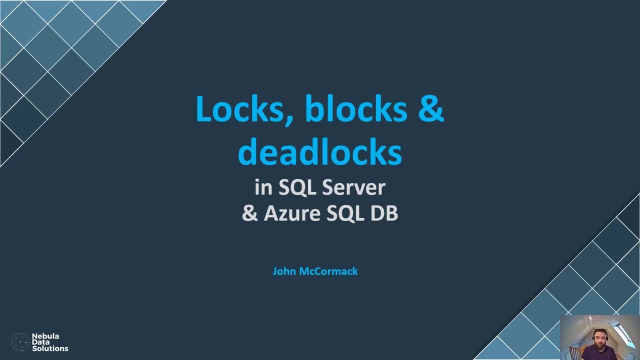 think that those terms are all pretty much the same. They know that something's going slow. They're probably describing blocking, which is one of the things that we're going to cover here, So let's have a click through and see what the difference is between. 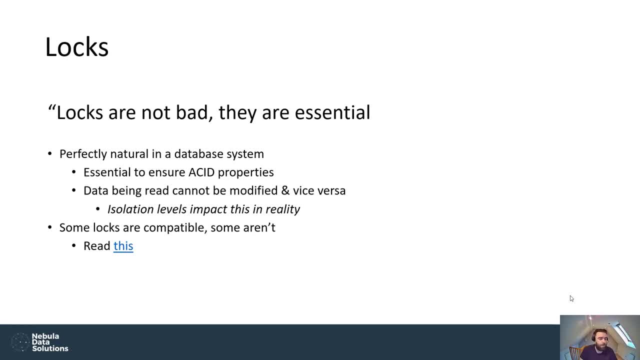 locks, blocks and deadlocks. So the first thing to say about locks is they're absolutely essential for a鬱DBMS system. So all the transactions need to request locks and be granted them. If we go over the SQL server's default settings, then if data is being Dallas-那么全 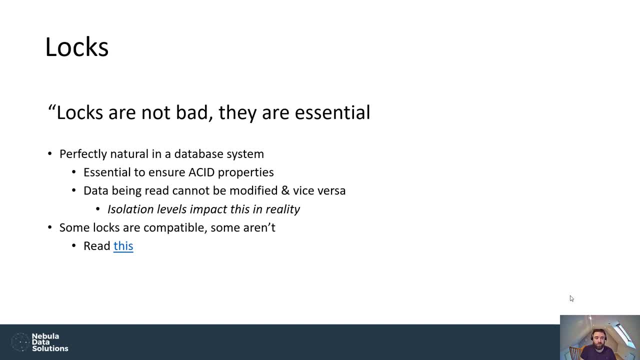 been read, then it can't be modified, and kind of vice versa. now there are ways round about this. some of them are really useful, some of them are are not ideal and really suboptimal. some lock types can happily coexist. so if you look at the link here on the presentation, which 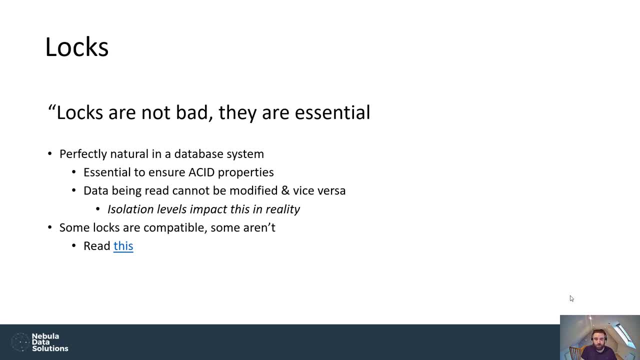 is in the, which is in the blog post, you can see a chart with all the different lock types and that can be requested in sql server and whether or not those lock types can exist happily alongside each other. some of them, however, are incompatible. so if they are incompatible, 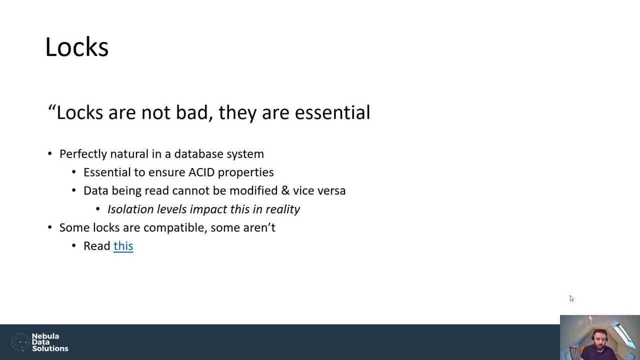 then what has to happen is the first transaction which has the lock has to complete before the next transaction can acquire the lock that it needs to get its business done. so that needs to be committed or rolled back. the full transaction has to happen, which is essentially part of what ACID means. it's an atomic transaction. 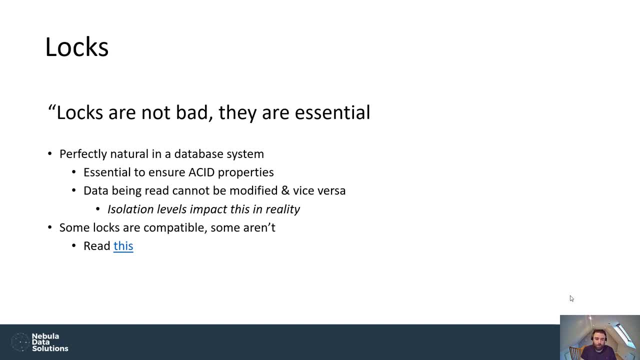 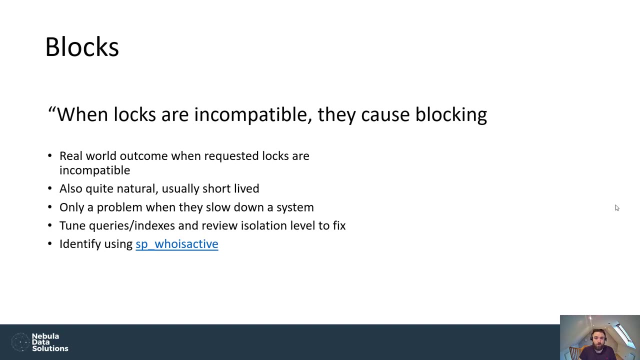 so if that hasn't fully completed, what's probably going to happen is that you're going to see delayed transactions, and that manifests itself in what we call blocking. so the person who told you about the problem, who said that can you clear all the deadlocks or the locks, whatever, 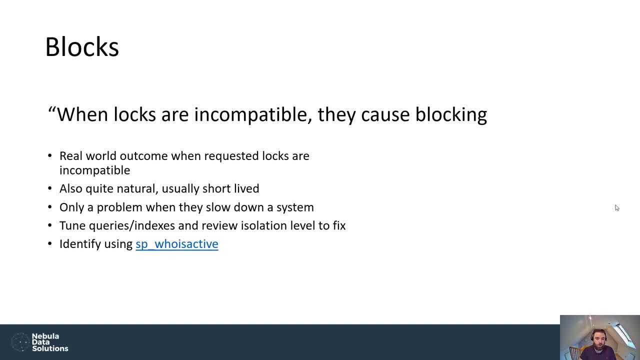 they were probably describing blocking, as I said, and blocking occurs when the locks are incompatible and have not completed. so most blocking is very short term and it's a result of concurrent transactions. so in the real world outcome of incompatible lock types being requested concurrently, it's usually only very short-lived, so we're talking microseconds or possibly milliseconds. 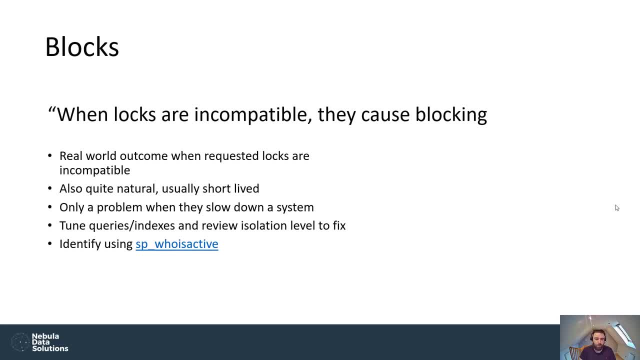 milliseconds, in some cases maybe into the low number of seconds. In most of these circumstances, that's not really a big problem. Okay, so the blocking is to be expected. It's a way that the SQL Server system is managing the consistency of the data within it. 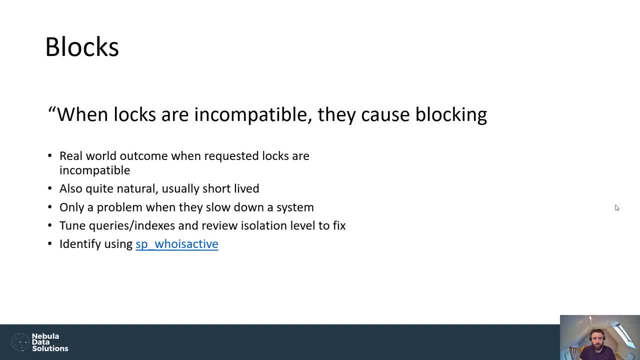 So the problem appears when blocking becomes like a really big issue is when the blocking isn't just for a matter of milliseconds or microseconds, but when it runs into seconds, large numbers of seconds and even minutes. So how do we fix this and how do we identify what is actually involved in the blocking? 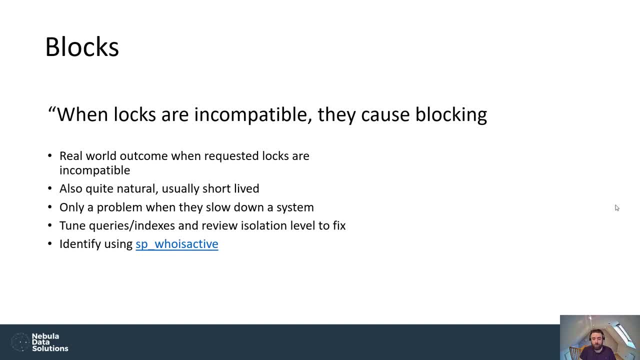 So I use SPWhoIsActive, which is a free of charge stored procedure written by Adam Mechanic. The link is on the blog post. It's available to download free of charge from his GitHub So you can inspect the code before you install it. 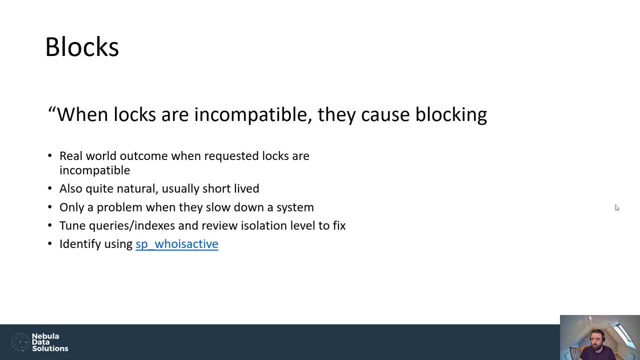 I believe it's perfectly safe. It's been used for decades now. It's constantly being updated, but it's been used by thousands of DBAs around the world. But if you want, have a read through the code before you use it. 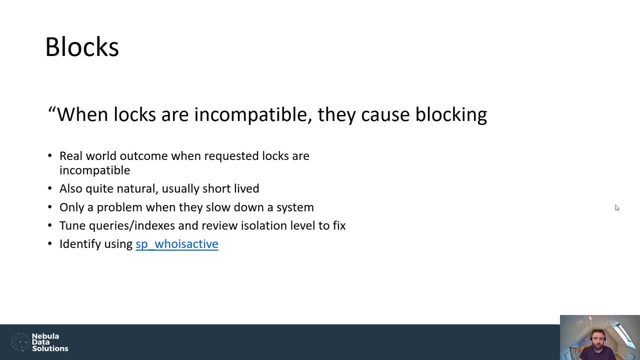 But it's an extremely useful stored procedure because it helps you get to the issue very, very quickly. If it's not just a one-off incident, if the same queries are showing up in your blocking time and time again, then you're going to have to look at tuning them. 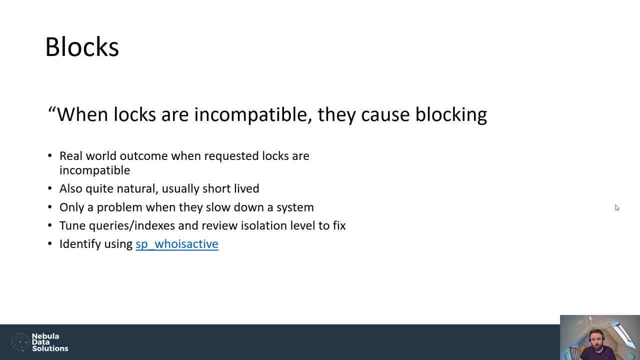 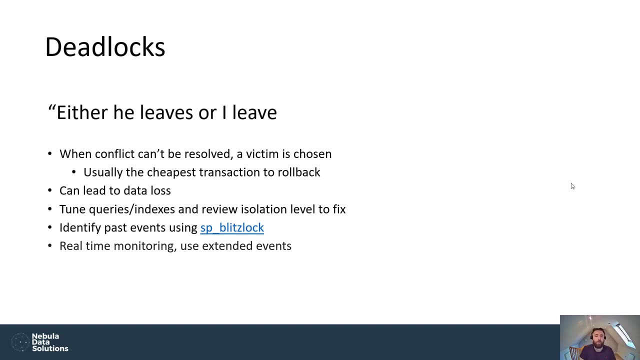 So whether that's tuning the queries, making sure that you have the appropriate indexes in place, and sometimes you may actually have to review the isolation level that you use. So the final thing is deadlocks, Deadlocks are. so I've said here: either he leaves or I leave. 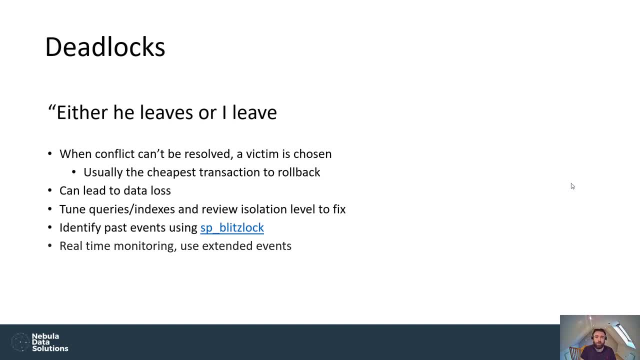 It's a situation where no one's going to give way, So SQL Server has to choose a victim. So what we mean by that is if there are two transactions which have incompatible lock types with each other, then the cheapest transaction to roll back is usually made the victim. 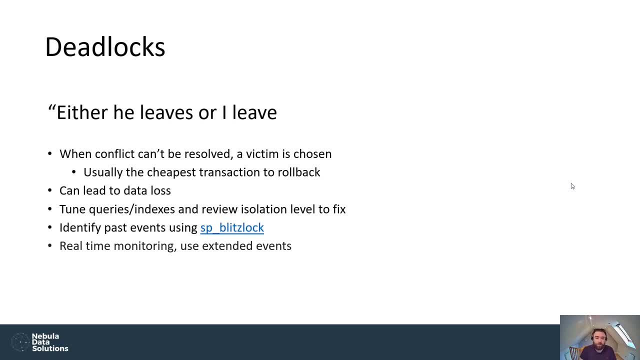 Now this can lead to data loss. So if the victim is doing some kind of insert, update or delete operation, then that whole transaction is rolled back, meaning that it's lost. If it was just reading data, then You would need to do the select again or get the application or report to run again. 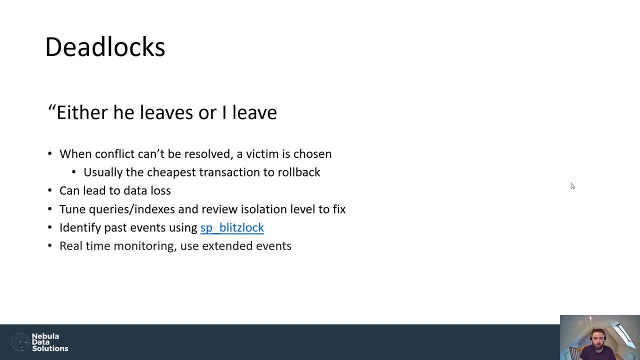 in order to get the data back that you need To identify past events, I use SP Blitzlock from Brent Ozar's first responder kit. Again, that's another completely free of charge stored procedure that you can review the code and install in your system once you're happy with it. 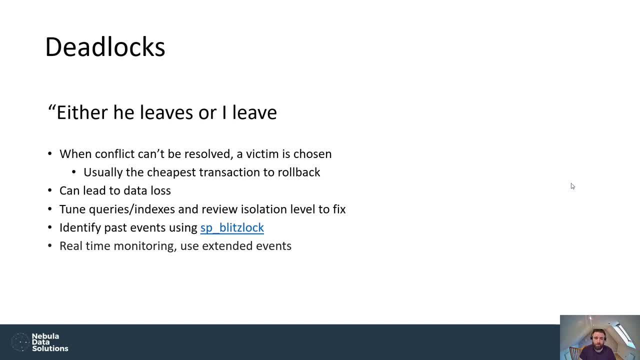 This is particular. It's really good if you want to look back over a fixed period of time, like: show me all the deadlocks in the last 24 hours and you can build up some patterns. If you're getting a lot of deadlocks, it may be the same groups or multiple groups of queries. 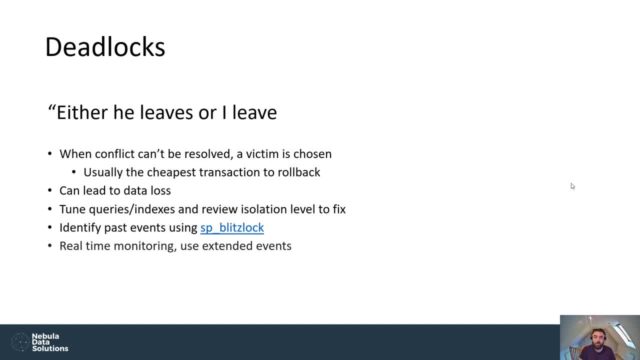 that are involved in these deadlocks and that will give you a start with what you need to go and start tuning and improving to avoid the future deadlocks. If you need more real-time information, then something like extended events is going to be the way that you're going to be able to get that out of. 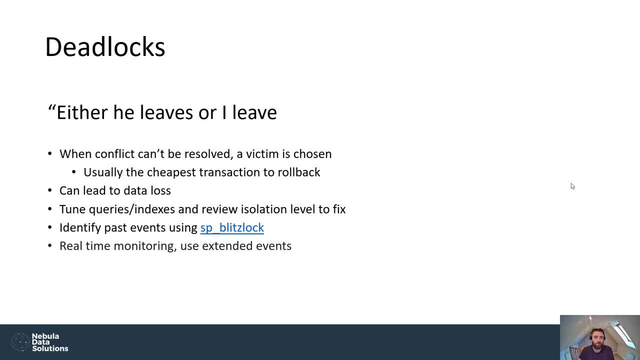 the system in a much more timely fashion. So now that we've covered the three terms of locks, blocks and deadlocks- or locking, blocking and deadlocking- hopefully we know how to use them correctly. now What I would like to do is show you an example of blocking, and that will also give us some 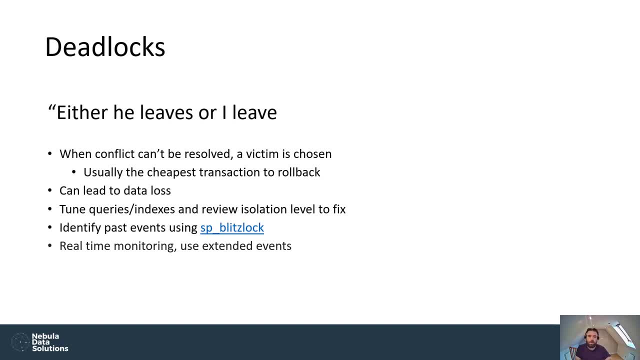 lock information as well. So I'm going to dive into Management Studio now to show you an example of blocking and we'll also look at the type of locks that are requested that have caused the blocking. So let's have a look at that using the examples that are listed on the blog post. 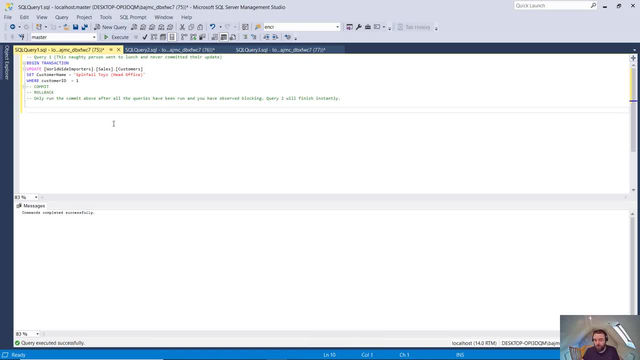 So here we are in the first query. This should have been a really simple query. The person wanted to update the name of a customer to Spintail Toys Head Office. We'll look at the next tab before we run that one. So it's currently called Spintail Toys HO. 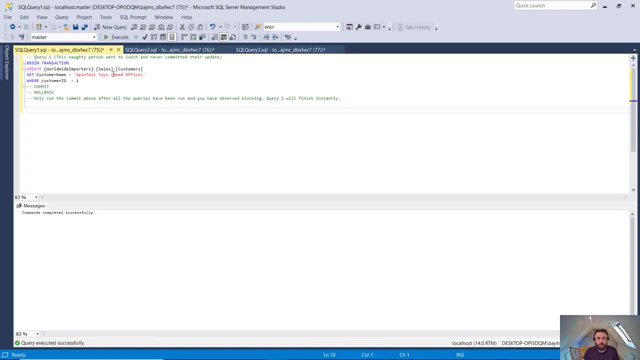 So all they want to do is just expand that HO to say Head Office, just to make things a little bit clearer when it comes up in the application. So they go to run the transaction. Now they use a begin transaction, which means that it won't automatically commit. 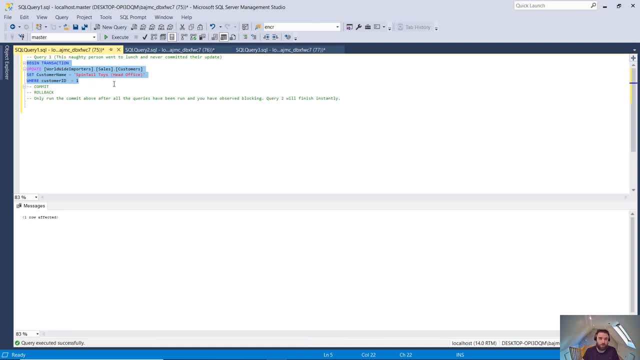 So we have an open transaction. It went through immediately, so normally you would be thinking: well, that was an immediate transaction, It won't be blocking anything because it's completed. But the fact that we haven't committed it specifically means that it's open and that 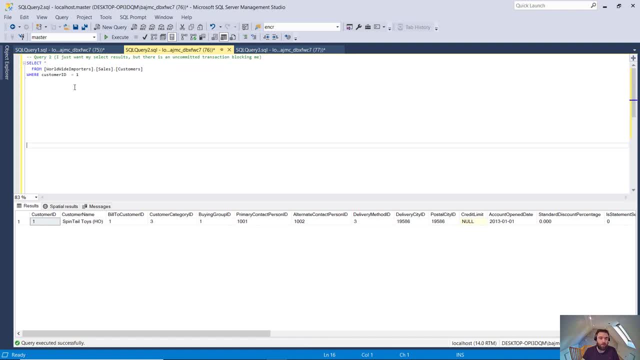 it should ideally cause some blocking in here. So here we are in query two and we just want to read all the customers, or rather just the customer, all the details of customer ID one. If we run this through then we can see that we're not getting the data back that we would. 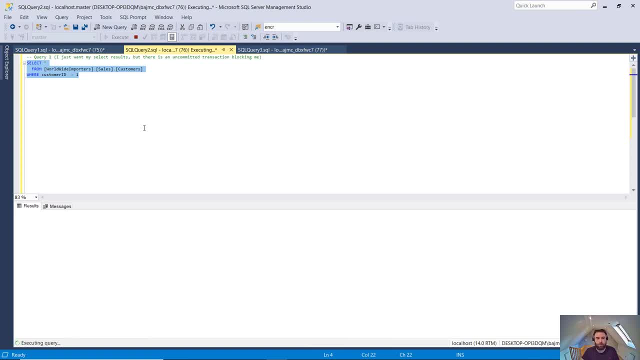 hope It's only looking for one row. it's using the ID value. it should be extremely quick, but something is stopping this, So in most applications you might see a default timeout of something like 30 seconds. The users would be expecting this to return almost instantly. 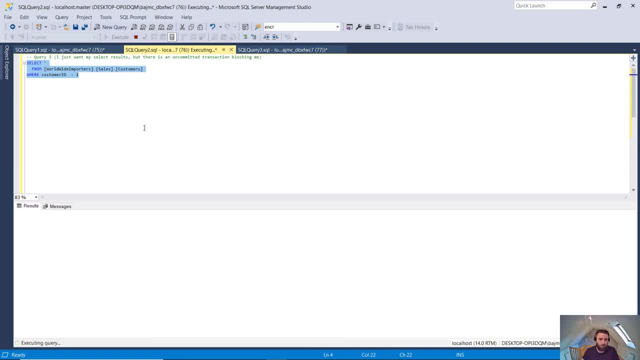 So once they're waiting for a few seconds, they think something's not quite right. the system's slow, and when they hit the 30-second mark, it may even prompt an error on their screen. So you're getting the report that there's slowness in the database, and what's the issue? 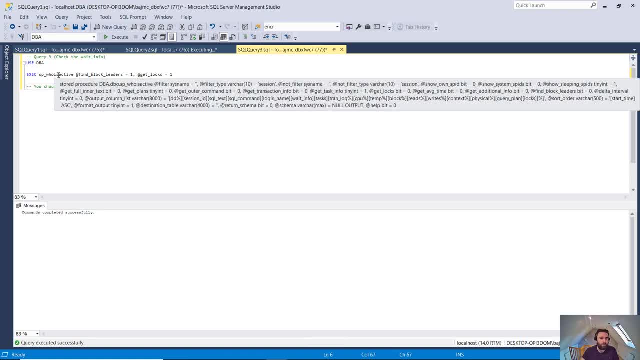 So you come in here and you want to run the transaction. You want to run this sp-who-is-active that I mentioned earlier, and you want to run it with the find-block-leaders and the get-locks parameters. Find-block-leaders is extremely handy if there's loads of blocking going on all over the place. 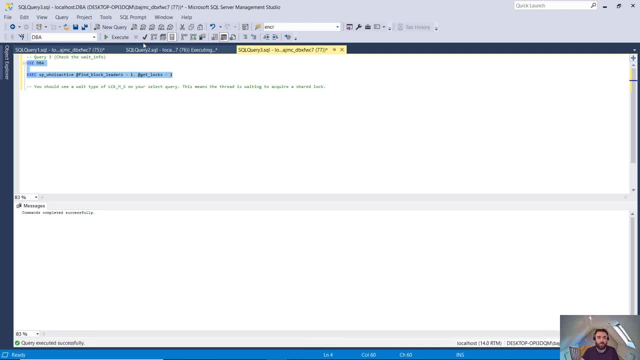 It will let you know which transaction is at the head of that and sometimes getting that killed if that's indeed necessary, will clear the rest of the blocking And the get-locks. just shows you which transactions are sorry, which locks are being requested. 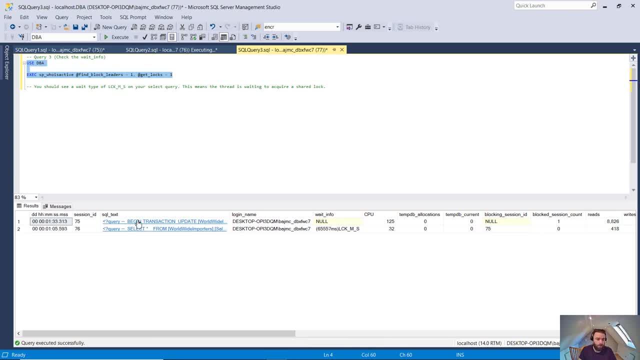 or taken At any point in time. So we can see that this begin transaction here that started one minute 33 seconds ago and the select started one minute and five seconds ago. Okay, so it's kind of been blocked for the full one minute and five seconds because it. 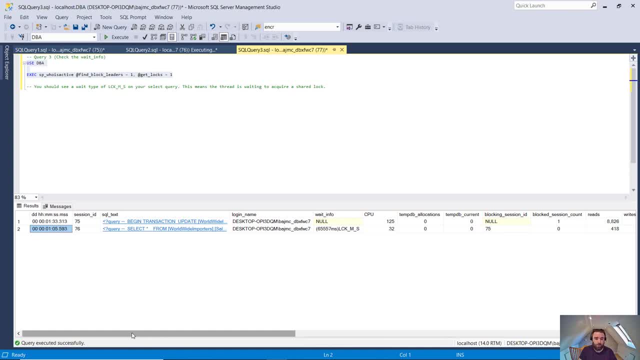 can't do what it needs to do, So all it wants here is a shared lock. Okay, that's what that lock type is, and you can easily Google that to find out what all the different locks are, What types are. but it can't get that shared lock at the moment, which means that there 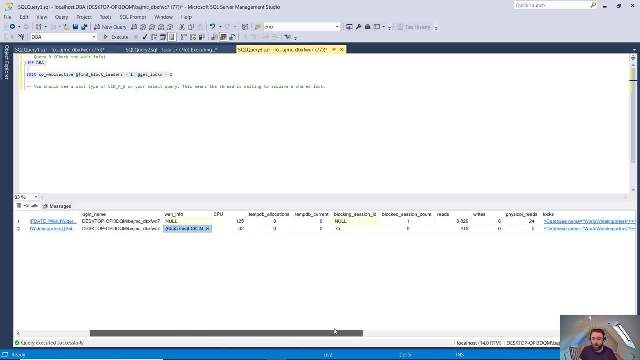 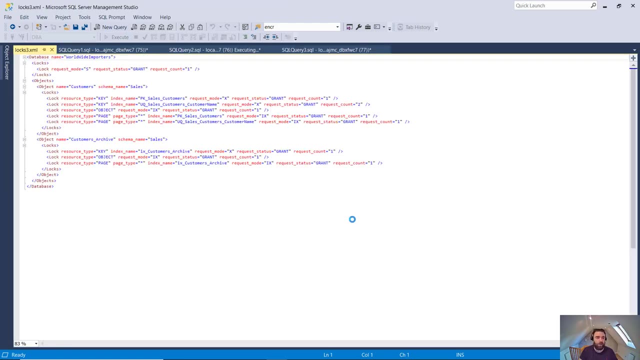 must be an incompatible lock type which is causing the blocking. So we know from in here that it's session 75 that's causing the blocking. So just scrolling along here and looking at this locks data, it's going to give us some data in XML format. 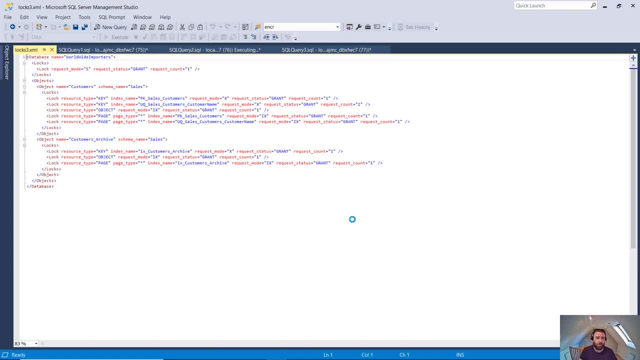 And it will show us all the locks that have been requested and granted in here. Now, here we can see, on this customer's table, on the primary key, there's been an exclusive lock granted. Okay, so there's been an exclusive lock granted there on the primary key. 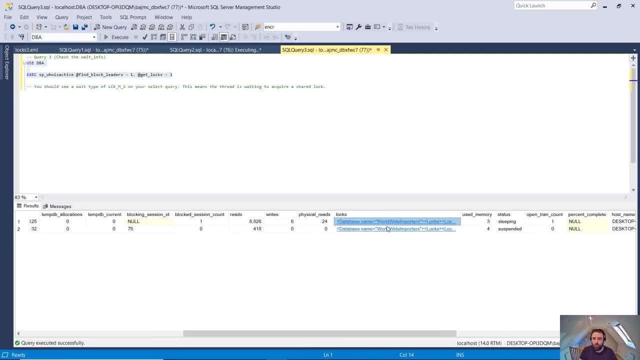 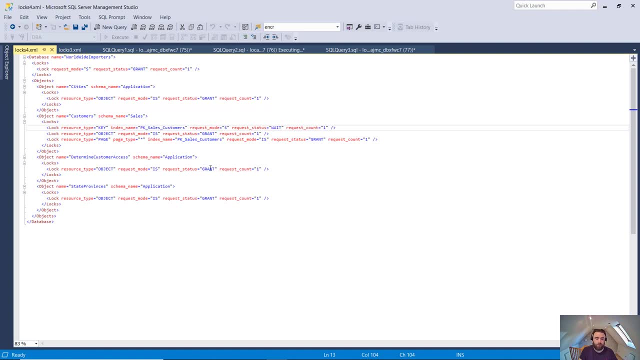 That's kind of the only thing that we need to know for now. If we want to look at the locks for the select query, there's a shared lock requested and it's going to give us some data in here, Okay, so that's kind of the only thing that we need to know for now. 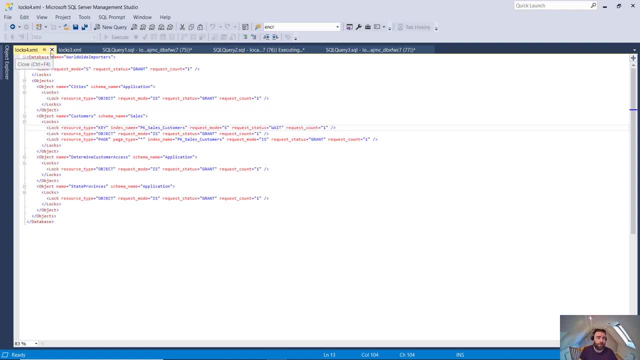 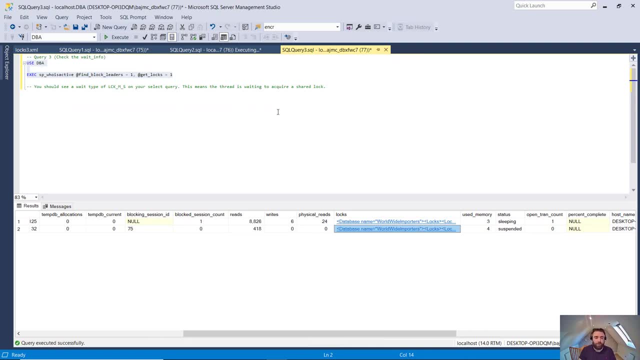 Okay, so that's kind of the only thing that we need to know for now. It's currently in the status of waiting and that's going to stay the same until something resolves here. Now, this isn't going to cause a deadlock, because it is expected that the first transaction will complete at some time, once someone takes the necessary action. 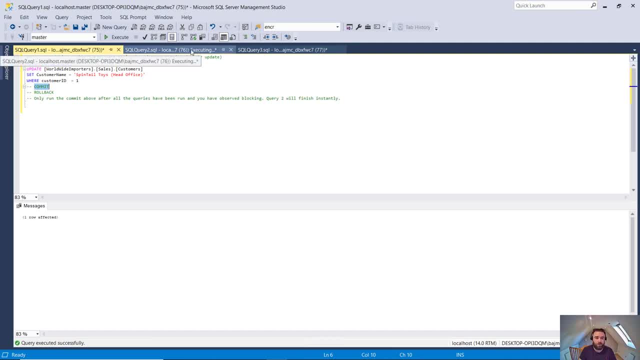 And in fact, if we do go in here and commit this, if you just look where that says executing in tab two, if I go in here and commit this, then you can see that in tab two it's immediately gone from executing to being completed. 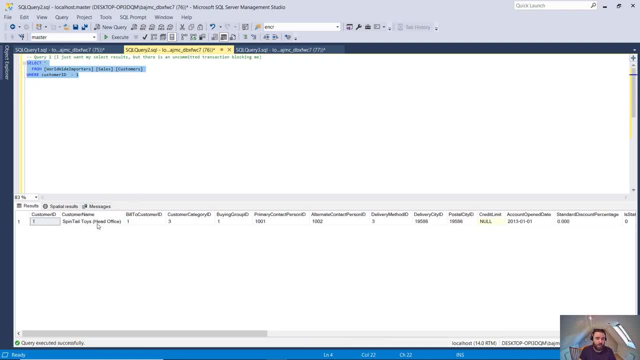 And, as you can see, it's gone from executing to being completed And, as you can see, it's gone from executing to being completed And, as you can see, it's giving us the up-to-date information. Spintail Toys with the full head office name. 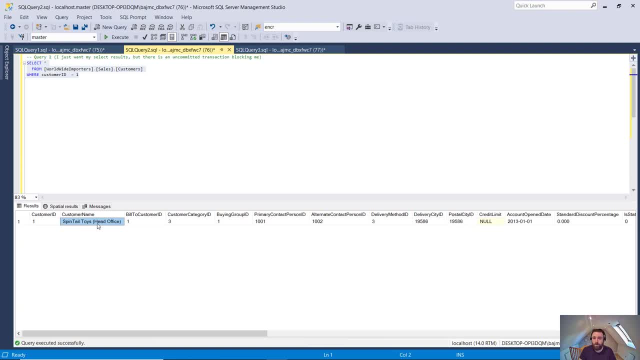 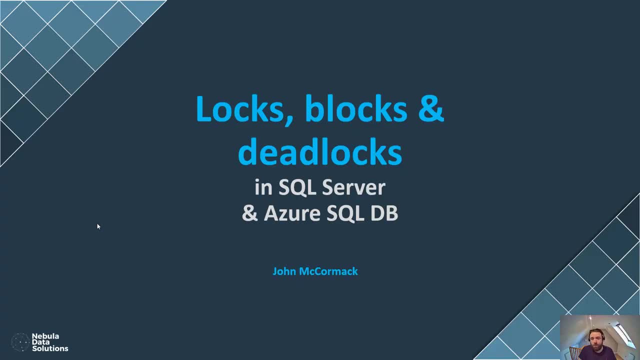 It hasn't given us any incorrect data, but it had to wait on that data being committed before it would allow the data to be selected. So that concludes the short video to accompany the blog post on locks, blocks and deadlocks. I hope that's been useful. 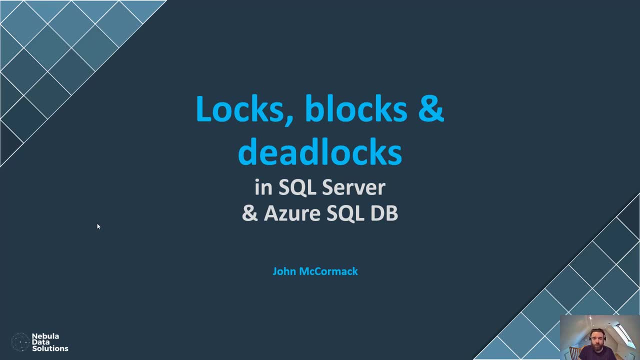 If you have any questions or comments, please leave them in the comments below. Thank you, Thank you.